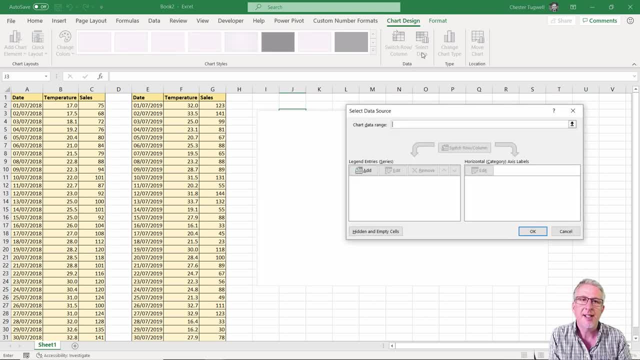 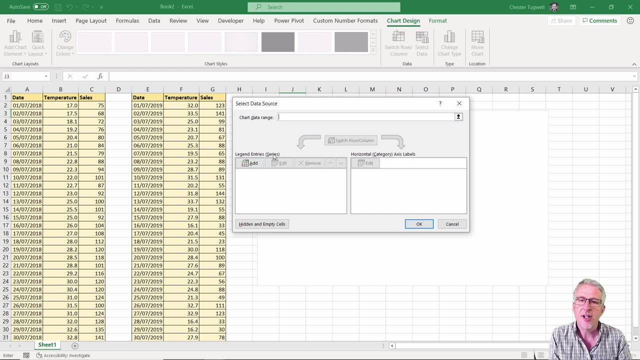 design tab on the ribbon and then I'm gonna make an empty scatter graph on the and I'm going to go to select data and in the select data source dialog I'm going to add a legend, entry or series. I'll click on add and I'm going to give. 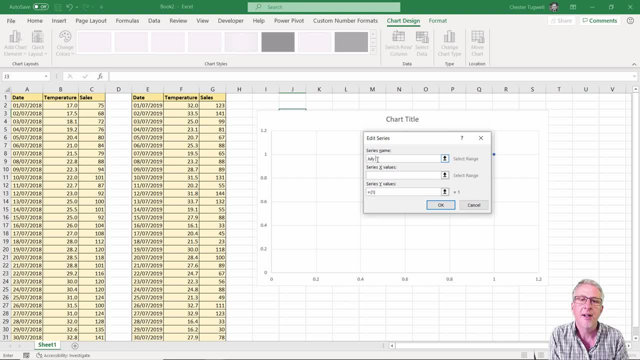 this series a name, so this first one I'm going to call July 2018. that's the series name. now, the X values, the horizontal axis. what I want on there is the, the sales, so I'm going to select the sales amounts for 2018. so it's control. 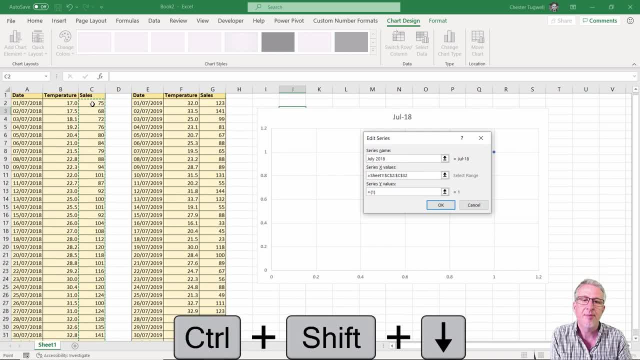 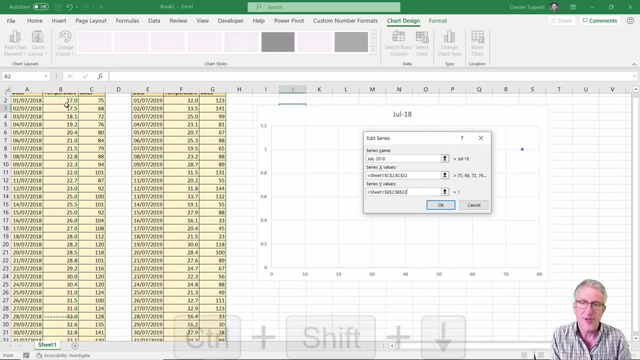 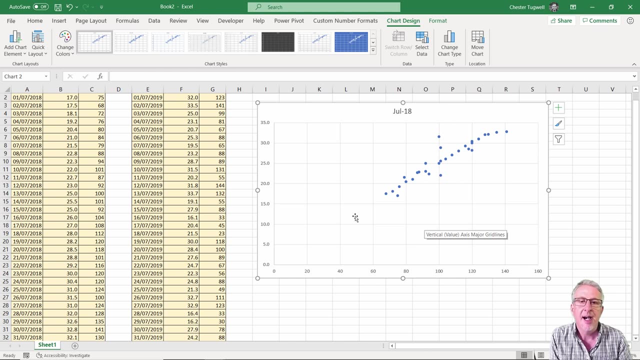 shift down arrow key to select down to the last consecutive value. and then for the Y values, I want that to be the temperature- highest temperature on the day. so again, control. shift down arrow key. okay, and if we just initially look at the values, that is plotted on a graph. so along the bottom we've got the sales. 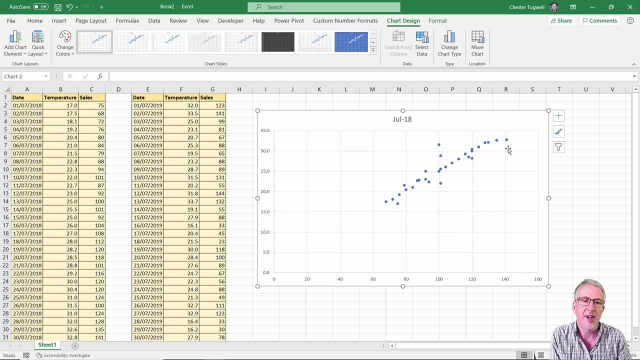 up the side. there we've got the temperature. we can see that there is a growth in sales as the temperature increases. so we need need to do the same for the 2019 data. so I'm going to go back to select data and I'm going to add: 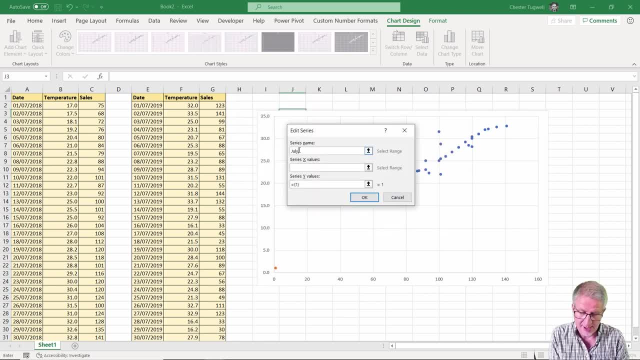 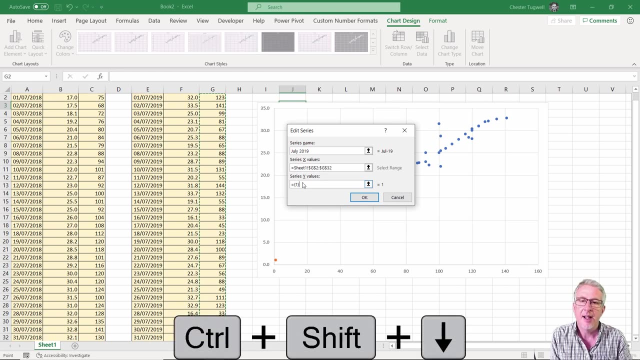 another series, and I'm going to call this July 2019. and again your X values. well, with my example, anyway, that's going to be horizontal axis, which is sales control- shift down arrow key. and then your Y values. it's going to be the temperature of the vertical axis control. shift down arrow key. click on, ok, click on. 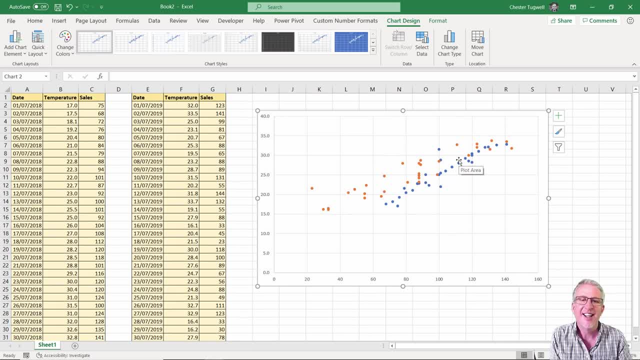 ok, and there we are. so slightly messier year in 2019. this one's a little bit neater, but nevertheless it does show the data. now I'm going to show a legend, so I'm going to go to my plus sign there show a legend and I think I'll show at. 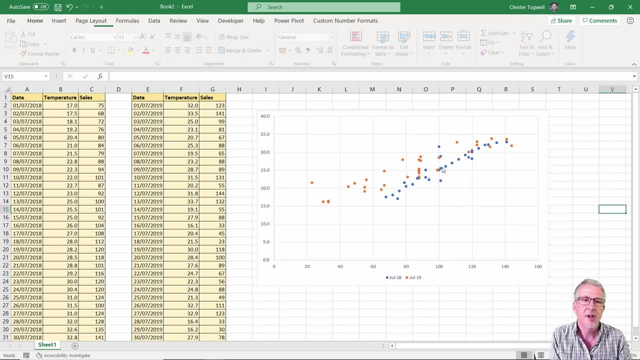 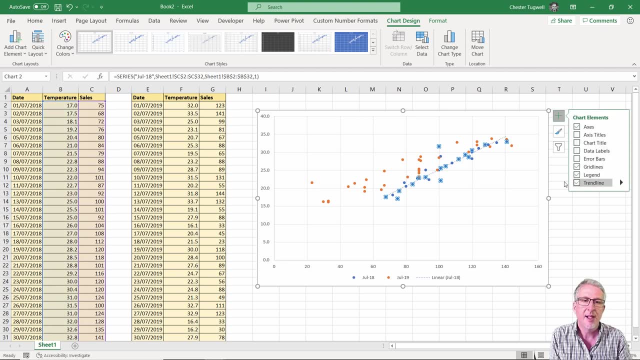 the bottom and I'm also going to show some trendline. so let's do it first. for the 2018 data, I'll show a trendline and I'm also going to show it for the 2019 data, so that neatly shows the trendline for.